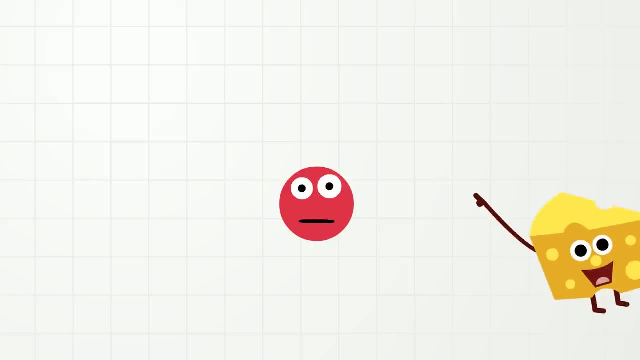 In a minute I am going to show you some more bananas, Bananas, And you are going to guess or estimate how many bananas there are. Bananas, You already said that. But first let us make sure we all know the numbers, from 1 to 10.. Let's all count to 10 out loud together, Ok. 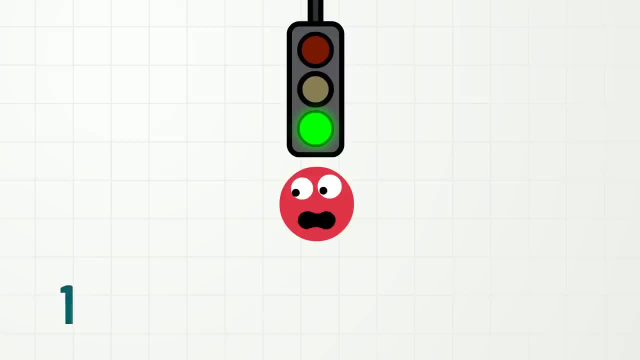 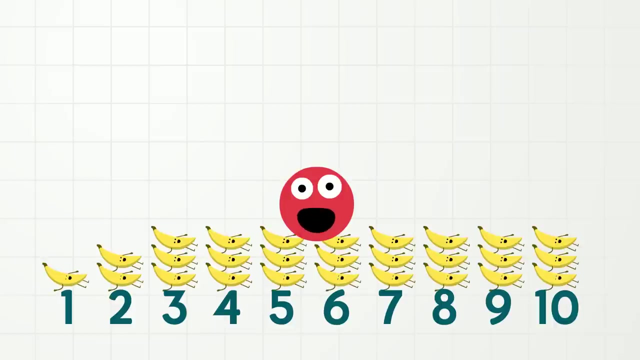 ready, Here we go. 1, 2,, 3,, 4,, 5,, 6,, 7,, 8,, 9, 10.. Good job. So these are all the numbers, or numerals, from 1 to 10.. And did you know that we can also show numbers using bananas? Oh, yes, we can. 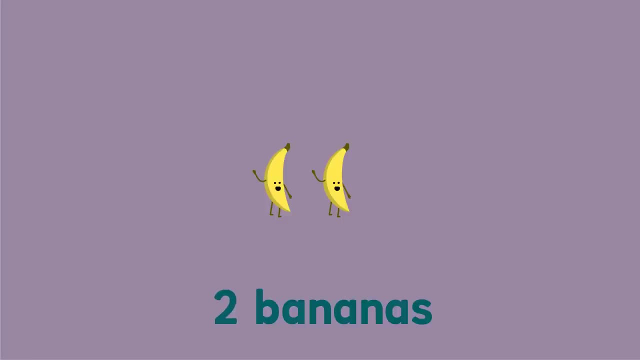 For example, This is what two bananas look like. This is what five bananas look like. This is what five bananas look like look like, and this is what 10 bananas look like. I will show you again. This is what two bananas look like, One- two. This is what five bananas look like: One- two. 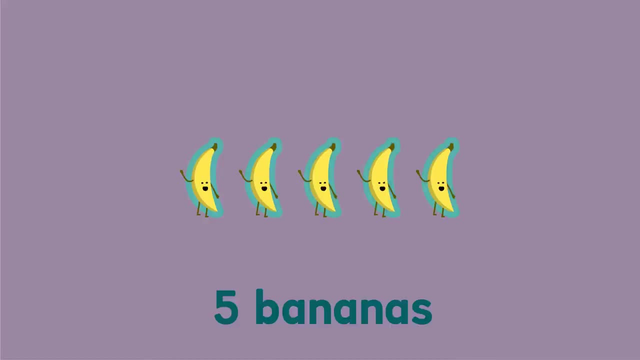 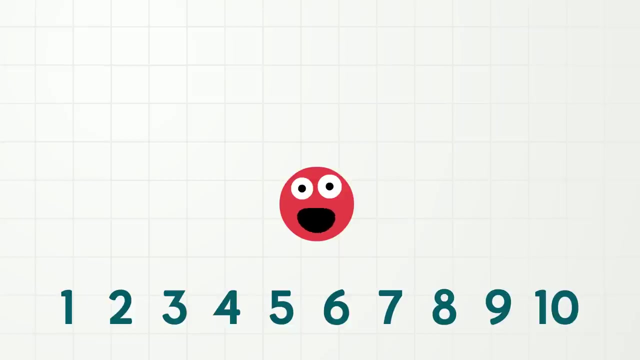 three, four, five. And this is what 10 bananas look like: One, two, three, four, five, six, seven, eight, nine, ten. So I am going to quickly show you some different bananas and I want you to estimate how many bananas you think there are. And 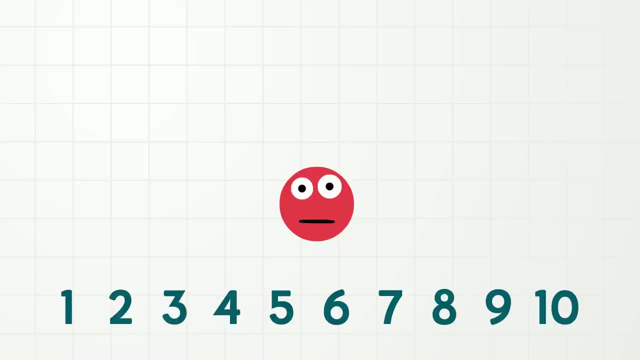 remember because you are estimating or guessing. it is okay if you don't know the exact number of bananas. Are you ready to see some bananas? Of course you are. Yeah, Here we go. Okay, that was a pineapple, not a banana. Who put their pineapple in there? 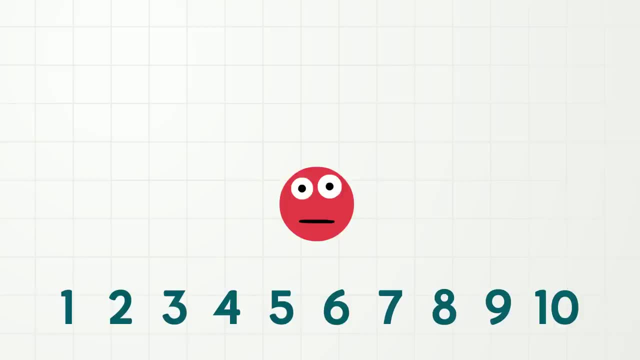 I did Sorry. Okay, let's try again. Ready, Here we go. So what was your estimate of how many bananas there were? Let's count and find out Bananas. I said bananas- One, two, three bananas, Remember. two bananas looked like this. So if we add: 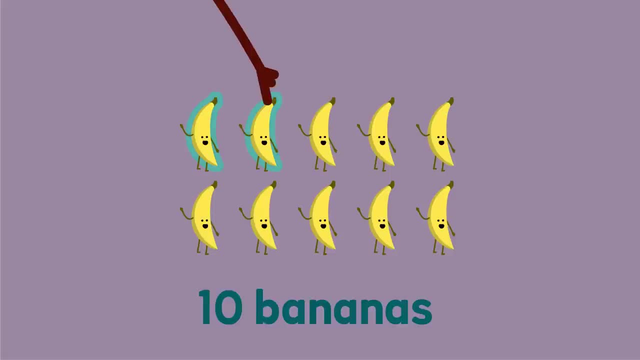 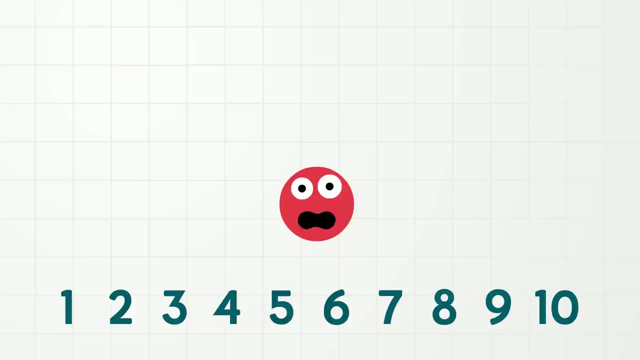 And this is what ten bananas look like: 1,, 2,, 3,, 4,, 5,, 6,, 7,, 8,, 9, 10.. So I am going to quickly show you some different bananas and I want you to estimate how many. 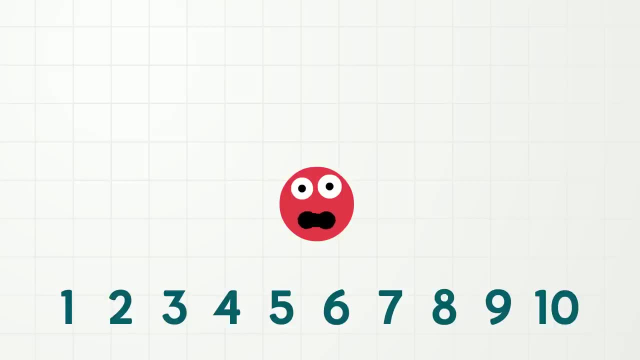 bananas you think there are And remember, because you are estimating or guessing, it is ok if you don't know the exact number of bananas. Are you ready to see some bananas? Of course you are. Yay, Here we go. 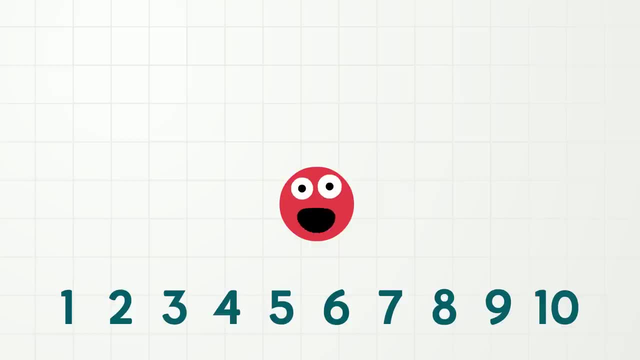 Ok, that was a pineapple, not a banana. Ok, now let's see how many bananas there are. Ok, that was a pineapple, not a banana. Ok, now let's see how many bananas there are. Who put that pineapple in there? 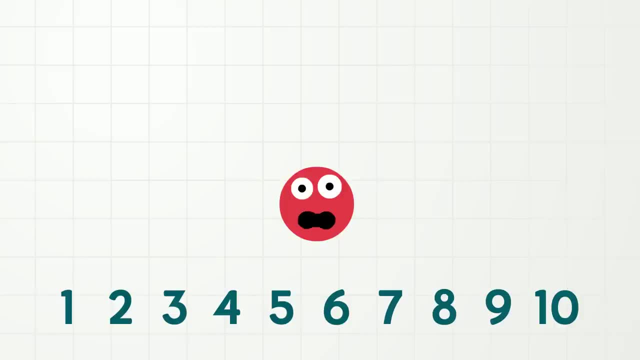 I did Sorry. Ok, let's try again. Ready, here we go. So what was your estimate of how many bananas there were? Let's count and find out Bananas. I said bananas 1,, 2,, 3 bananas. 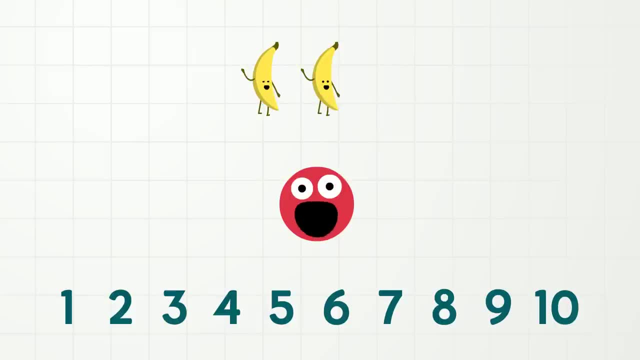 Remember two bananas? look like this. so if we add one more, we know that two plus one is three. Three bananas, Bananas. Ok, you did such a good job, let's take a quick break. Ok, that's enough. 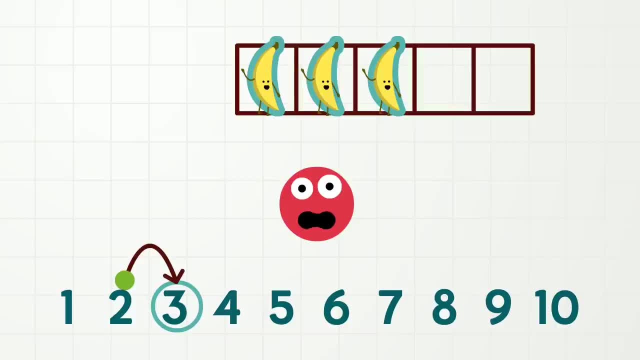 Now let us do some estimating again. with a different number of bananas Ready, here we go. So what was your estimate of how many bananas there were? Let's count and find out: 1,, 2,, 3,, 4,, 5,, 6,, 7,, 8,, 9,, 10,, 11,, 12,, 13,, 14,, 15,, 16,, 17,, 18,, 19,, 20,, 21,, 22,, 23,, 24,. 25,, 26,, 27,, 28,, 29,, 30,, 31,, 32,, 33,, 34,, 35,, 36,, 37,, 38,, 38,, 39,, 40,, 41,, 42,, 42,, 43,. 45,, 40,, 41,, 42,, 43,, 45,, 40,, 42,, 45,, 46,, 46,, 47,, 49,, 49,, 50,, 51,, 92,, 53,, 53,. 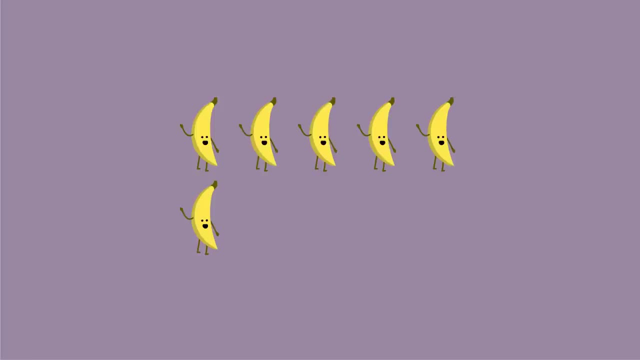 52,, 54,, 54,, 54,, 55,, 56,, 57,, 58,, 69,, 60,, 61,, 62,, 63,, 62,, 62,, 63,, 53,, 62,, 62,, 62,, 63, Gauss. 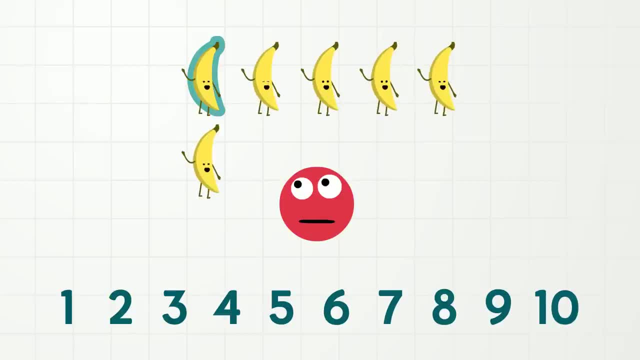 Party. Nice job. Then what happened? The highest number of bananas that were there is eight. This was because the highest number of bananas is less. This means that another number of bananas is less. About answers are left. So I had an顶 mistake here. 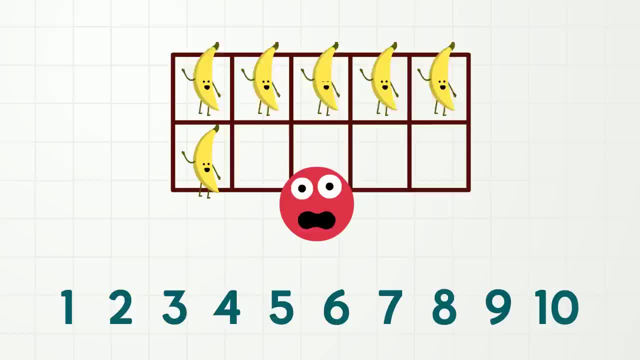 I said, the number cannot account for everything, So I had to risen the plan on another number of bananas. That's why I repeat: For example, if you add one more bananas, how many bananas could there be? 5 bananas look like this: 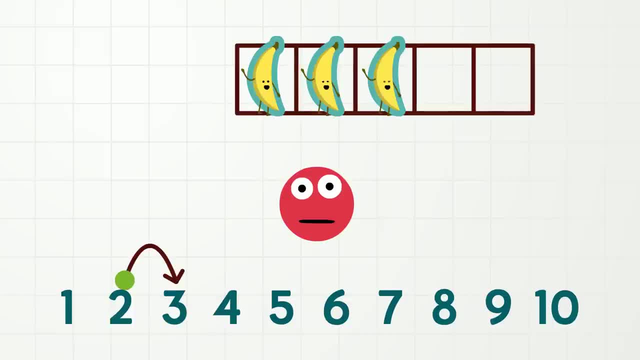 one and all five bananas by each. give yourselves four bananas. This is what? five And so one more. we know that 2 plus 1 is 3. Three bananas, Bananas. Okay, you did such a good job, Let's take a quick break. Okay, that's enough. Now let us do some estimating again. 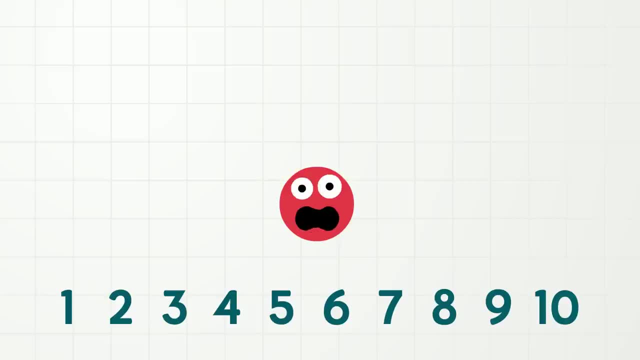 with a different number of bananas Ready. Here we go. So what was your estimate of how many bananas there were? Let's count and find out: One, two, three, four, five, six bananas. Remember that five bananas look like this. So if we add one more, we know. 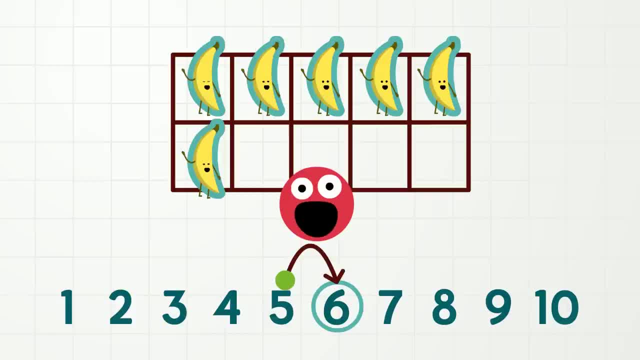 that 5 plus 1 is 6.. Six bananas- Bananas. If you estimated that there were six bananas, good job. If you estimated that there were five bananas, also good job, Because five is close to six. Want to know something? Of course you do. 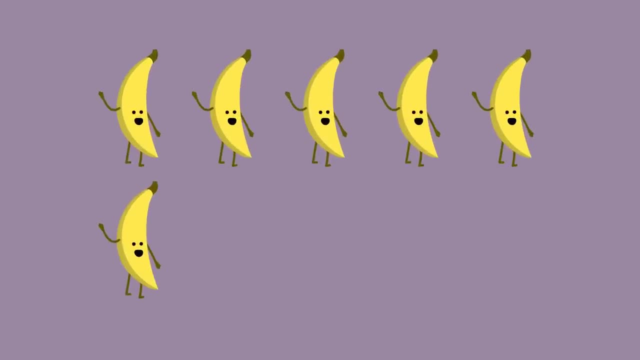 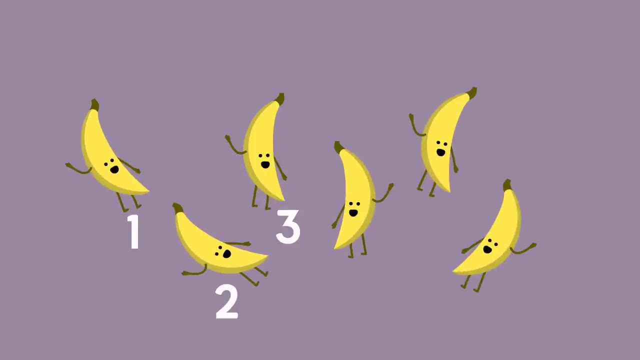 Six bananas don't always look exactly like this. They could look like this, and there would still be six. They could also look like this, and there would still be six. They could also even all have funny hats, and there would still be six. Okay, let us do some estimating. 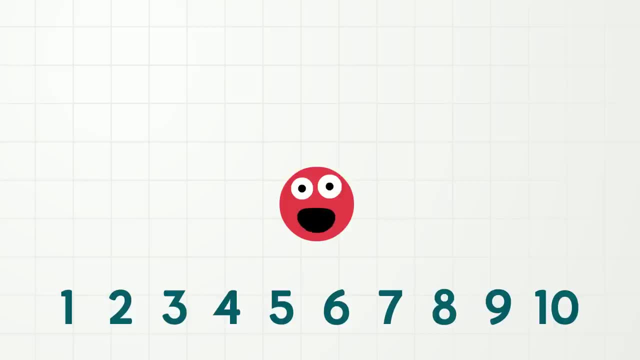 one last time with a different number of bananas Ready. Here we go. So what was your estimate of how many bananas there were? Let's count to find out: One, two, three, four, five, six, seven, eight bananas. Remember that five bananas look like this: 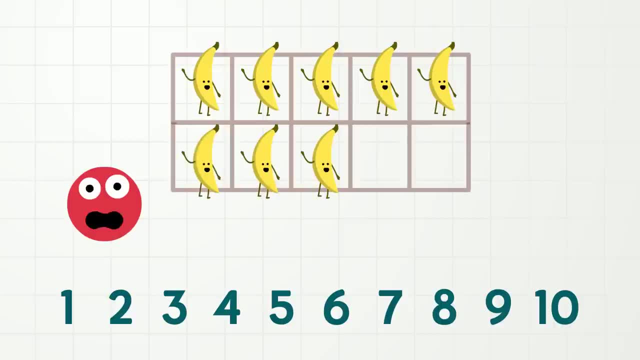 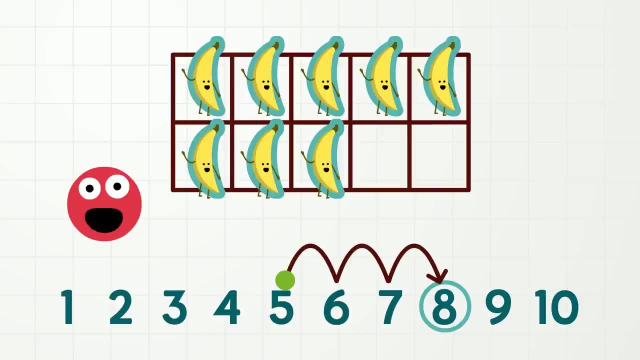 So if we add three more, we know that five plus three is eight, Eight bananas. But maybe you estimated a different number and that's okay. For example, remember that ten bananas look like this: So if you take away two bananas, we know that ten. 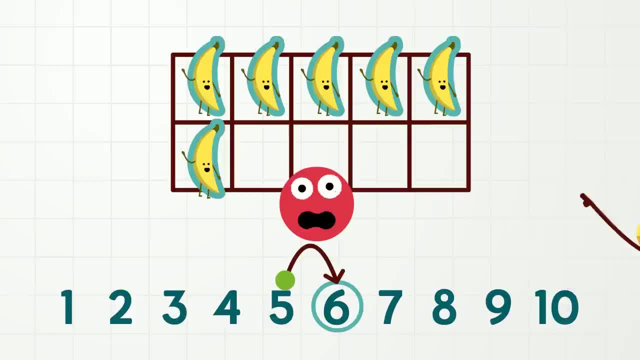 six, Six bananas, Bananas. If you estimated that there were six bananas, good job. If you estimated that there were five bananas, also good job, Because five is close to six. Want to know something? Of course you do. Six bananas don't always look exactly like this. They could look. 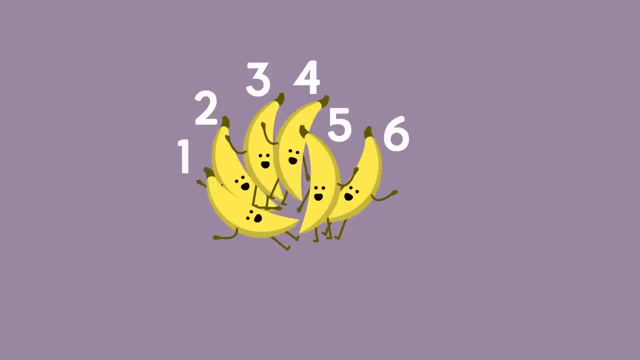 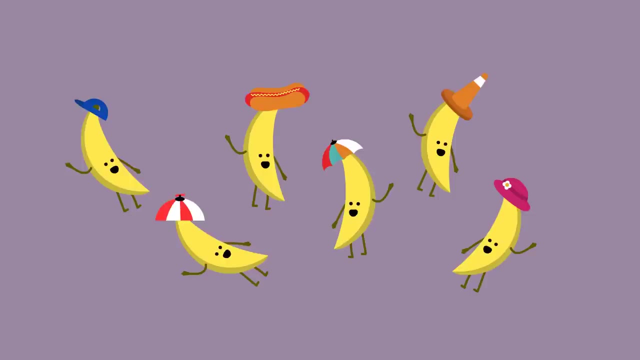 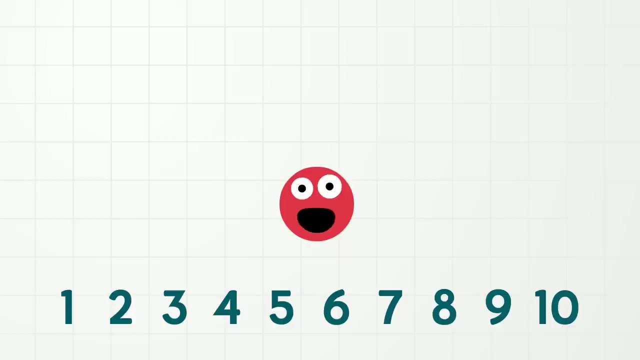 like this, and there would still be six. They could also look like this, and there would still be six. They could also even all have funny hats, and there would still be six. Okay, let us do some estimating. one last time, with a different number of bananas Ready. Here we go. So what was your? 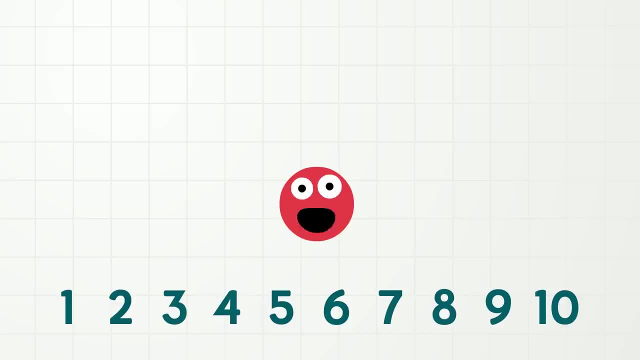 estimate of how many bananas there were. Let's count to find out 1,, 2,, 3,, 4,, 5,, 6,, 7,, 8 bananas. Remember that five bananas look like this. So if we add three more, 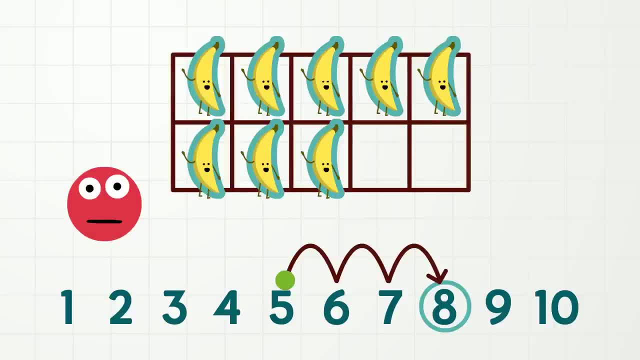 we know that five plus three is eight, Eight bananas, Bananas. But maybe you estimated a different number, and that's okay. For example, remember that ten bananas look like this: So if you did that, you would know that there were six bananas. So if you estimated that there were, 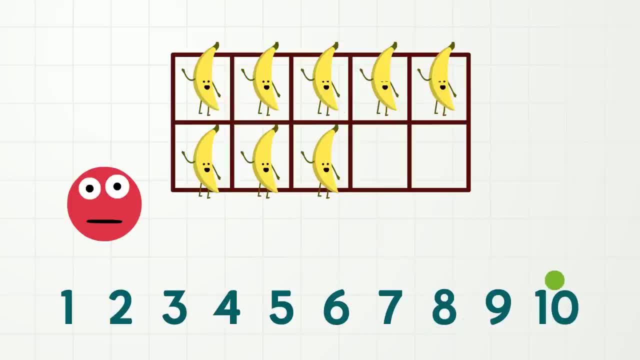 eight bananas, you would know that there were six bananas. So if you did that, you would know that there were six bananas. So if you did that, you would know that there were six bananas. So if you take away two bananas, we know that ten minus two is eight Eight bananas. Bananas. If you estimated, 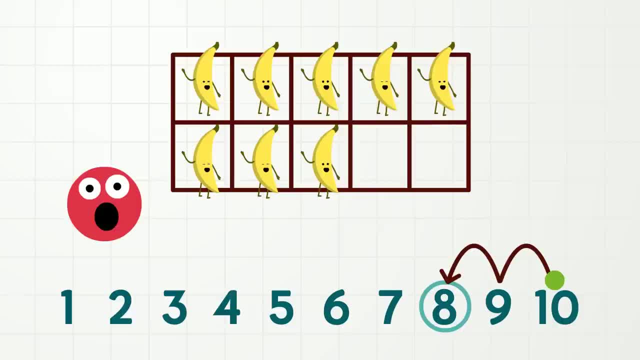 that there were eight bananas, good job. If you estimated that there were five or ten bananas, also good job, because five is kind of close to eight, and ten is also close to eight too If you estimated that there were 100 bajillion triple bananas. that is not so good. 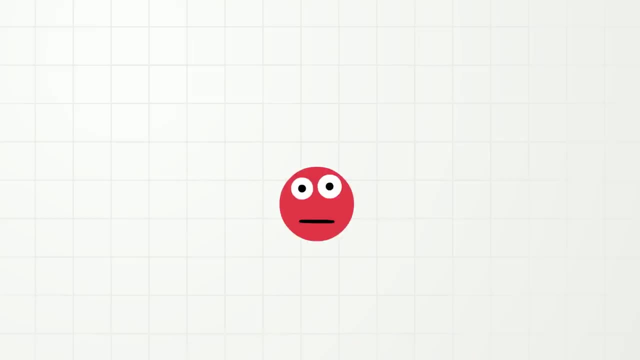 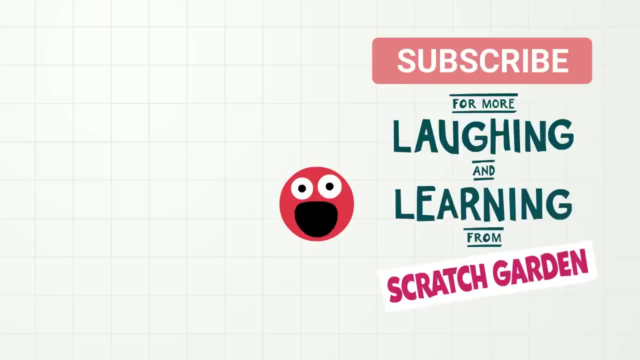 because that is not even a real number. Okay, that is all the time we have today for estimating. Don't forget to subscribe to our channel for more laughing and learning from Scratch Garden. And did you know that we have other videos on counting And even some other videos with bananas? 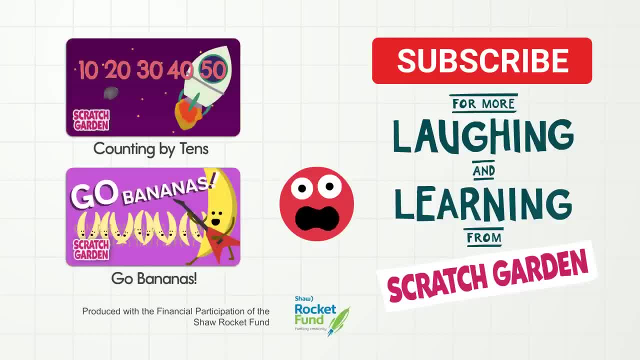 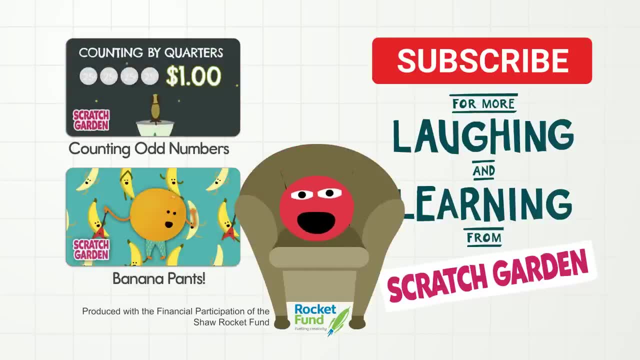 No, it's true. In fact, I estimate that you will soon watch one of our banana videos, very soon. Okay, bye for now. Bananas.